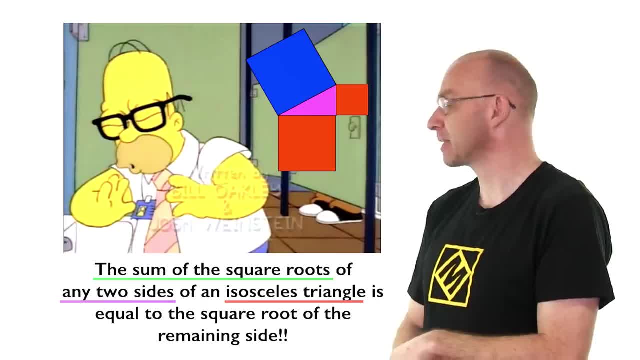 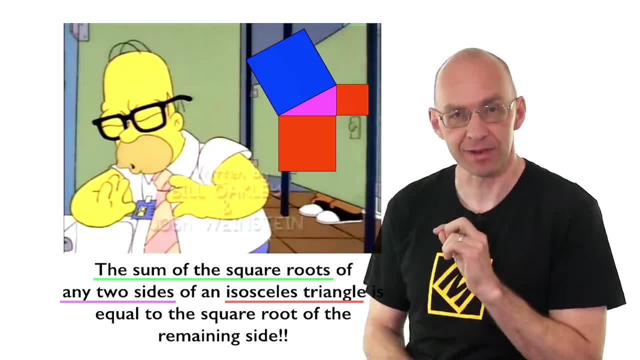 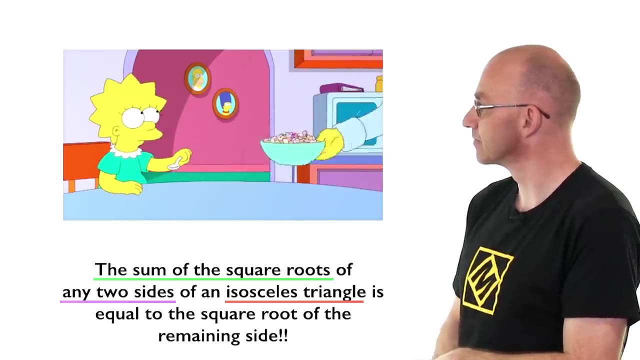 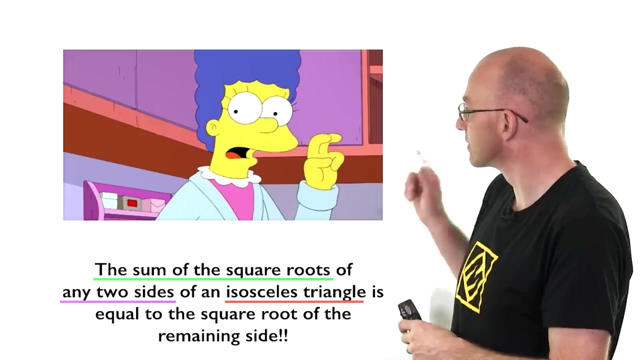 So maybe he actually did not have. he did not have Pythagoras in mind. Maybe he learned it somewhere else- And there's actually another Simpsons episode that gives you a bit of a hint where he may have learned it. Ooh, there's new marshmallows in the Belfast charms. No, no, that's Bart's cereal. It's the only way I can get him to take his vitamins. 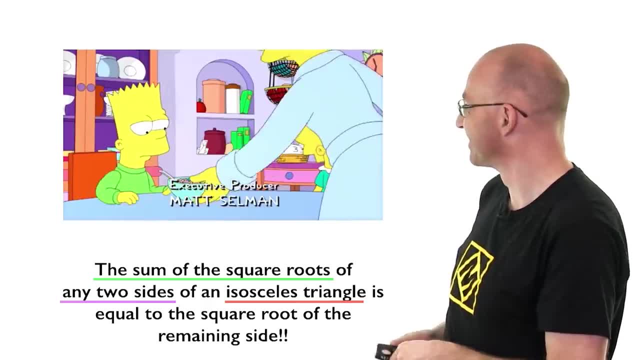 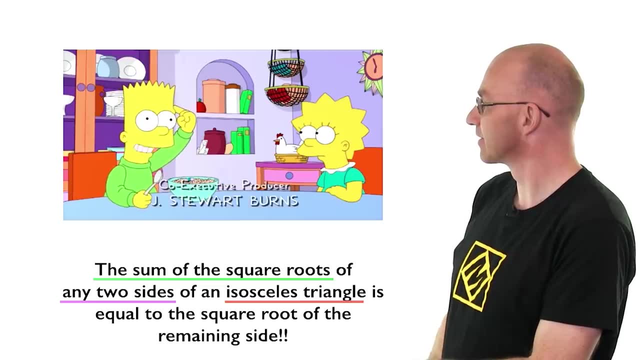 Yep, The sum of the square roots of any two sides of an isosceles triangle is equal to the square root of the remaining side. That's not right. Yes, it is. They're my lines as a scarecrow and the Wizard of Oz. 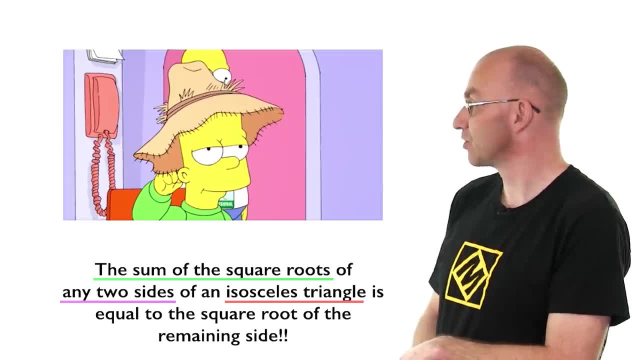 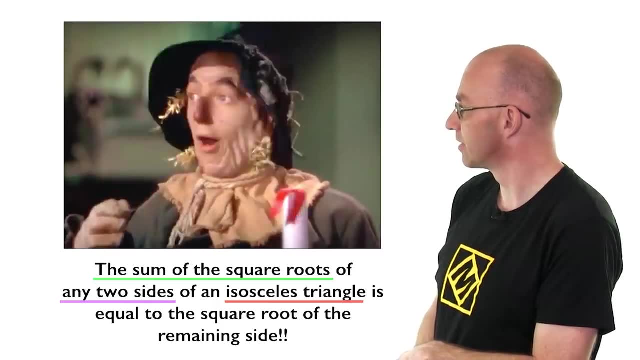 Hmm, the scarecrow and the Wizard of Oz. Actually, if you go to the movie and you find the scarecrow, The sum of the square roots of any two sides of an isosceles triangle is equal to the square root of the remaining side. 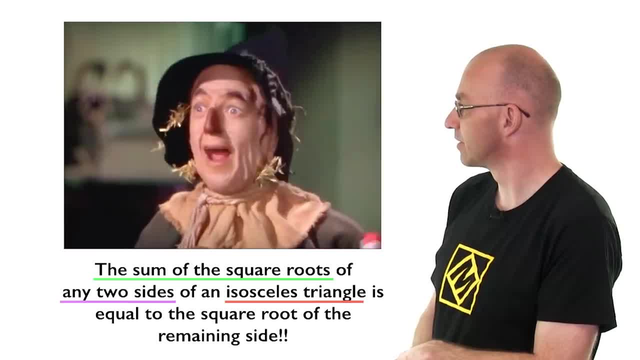 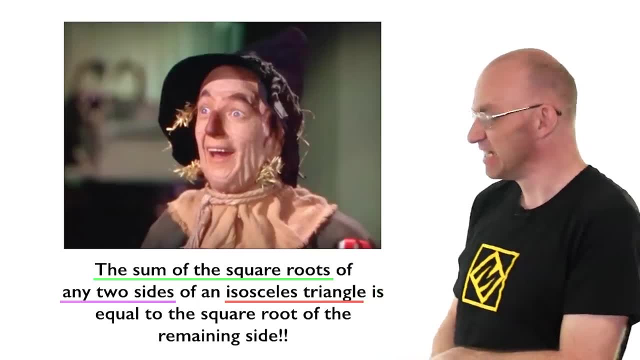 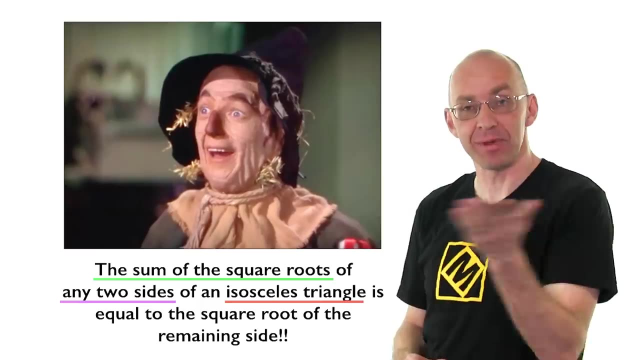 Oh joy, rapture, I've got a brain. So he says this after he's got a brain: He's got the brain right. Looks like he got a bad deal. He got a bad deal, yeah, But maybe not. Maybe he's right, you know. 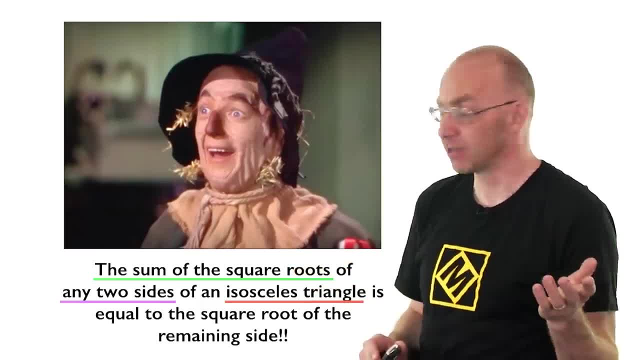 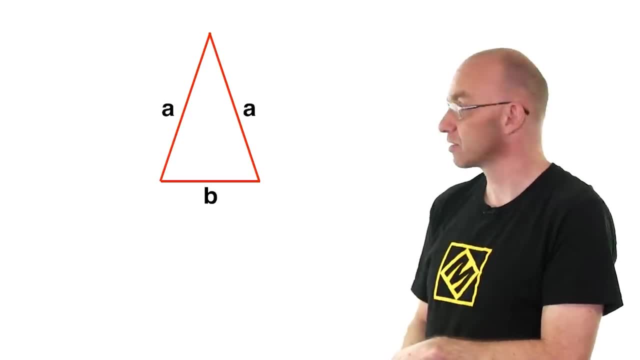 Just because this sounds similar to Pythagoras doesn't mean that it has to be. You know, it might still be correct, right? So let's have a really, really close look. Maybe it is correct, right? So here's an isosceles triangle. So what makes a triangle isosceles? 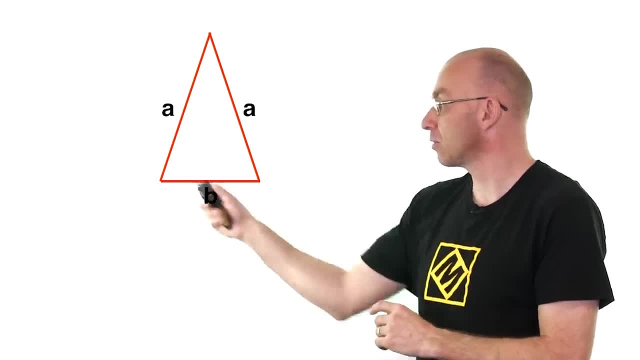 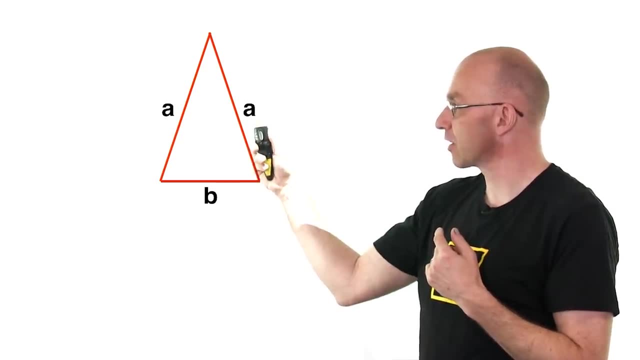 You've got two sides that have equal lengths, okay, Or two angles here are the same, Alright. now what does he say? He says: if I do the square root of this and add to it the square root of that, you get the square root of this. 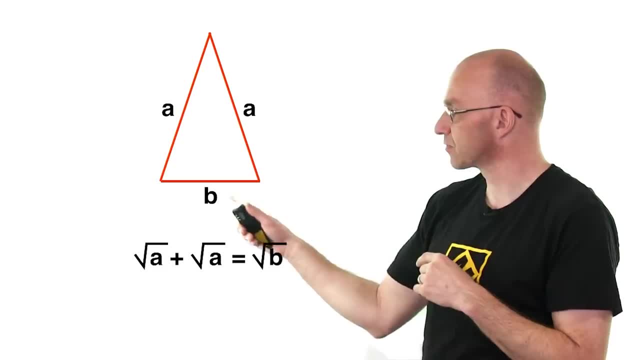 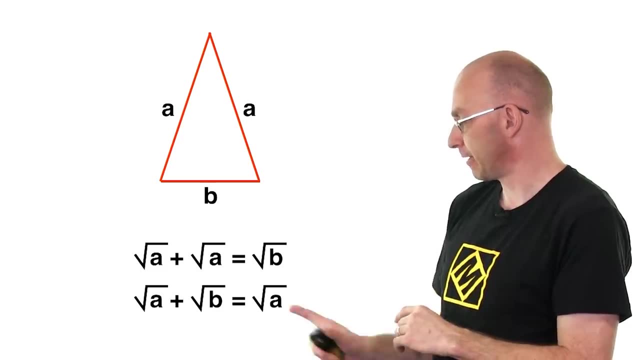 But he also says: you can do this with any two sides. So I should also be able to kind of start: square root of this plus square root of that is square root of that. So let's also write down that one here. Now have a look at this one here. 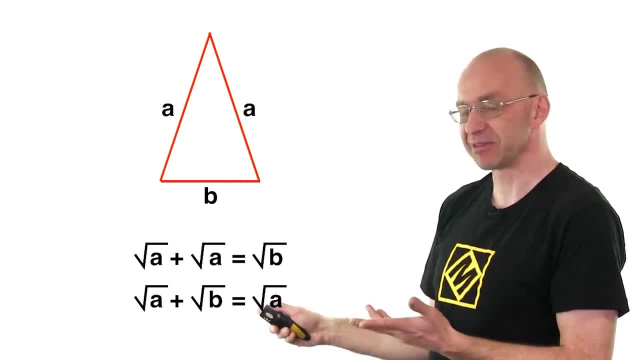 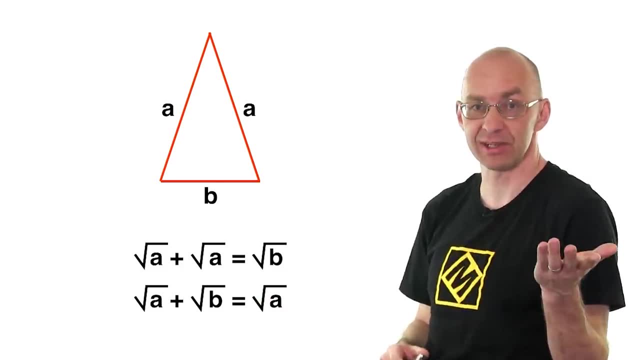 Well, that doesn't look right, Well, it's okay. but I mean you've got two times the square root of A on two sides of the equation. So what can we do? We can just cancel it out. So we cancel it out goes, and then what's left over is square root of B is equal to 0,. 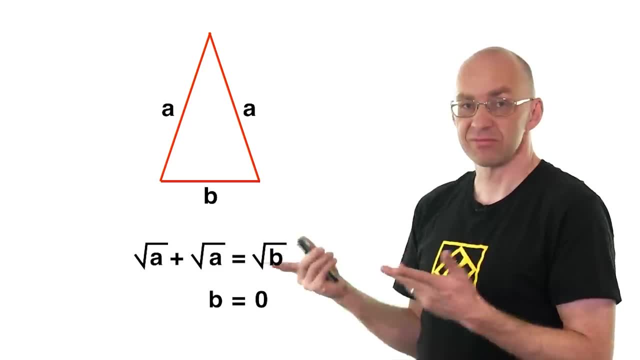 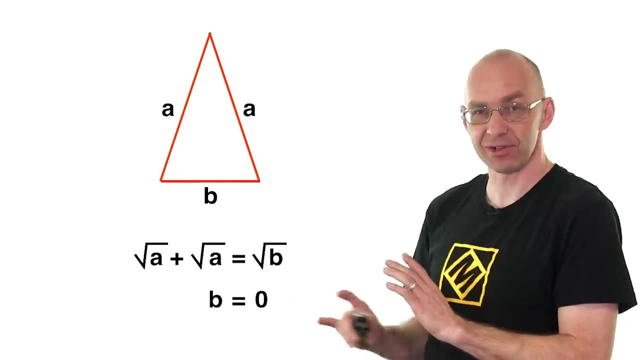 which means that B is equal to 0.. No, So you get a line, You get a line right. I mean, maybe you consider this as an isosceles triangle, but usually not right. So I mean there's definitely something that's not quite right. 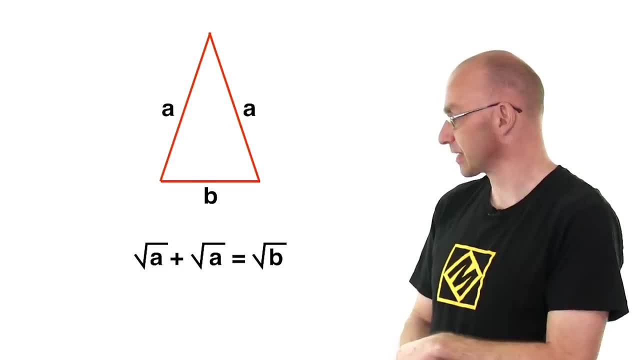 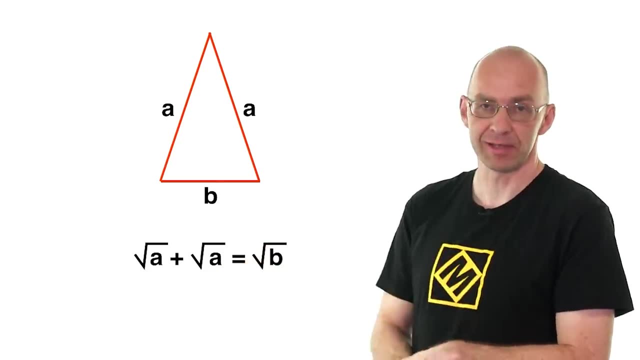 But let's just forget about this any-two-sides business, okay, Maybe just this was meant right. So square root of A plus square root of A is equal to square root of B. Maybe he meant that one right? Well, let's just have a look. 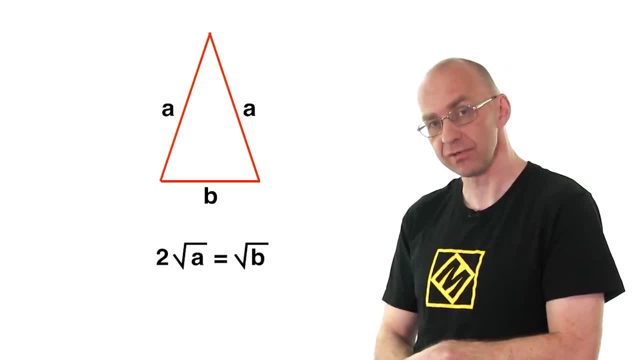 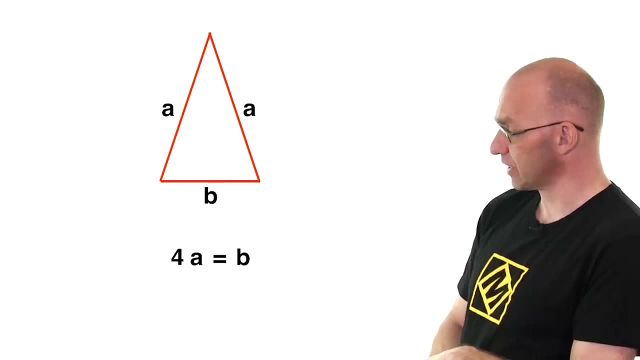 So what we do is we pull those two things together, So it's 2 times square root of A. What do we do now? Pretty obvious: We square to get rid of the square roots. So we get this one here And now we'll have a really, really close look at it. 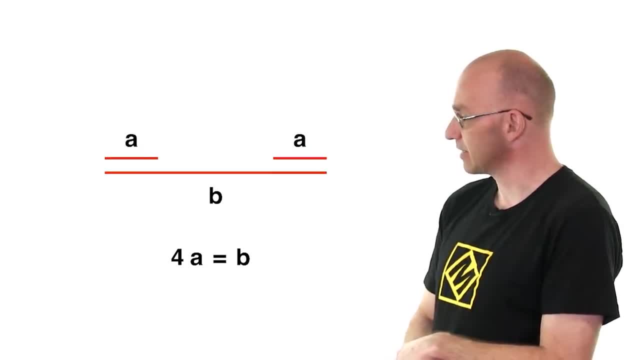 And actually we can do this in pictures here. So what this says is: we've got like A and we've got A, and B is four times as long as A, And it's pretty obvious. you can't make any triangle out of anything like this, right. 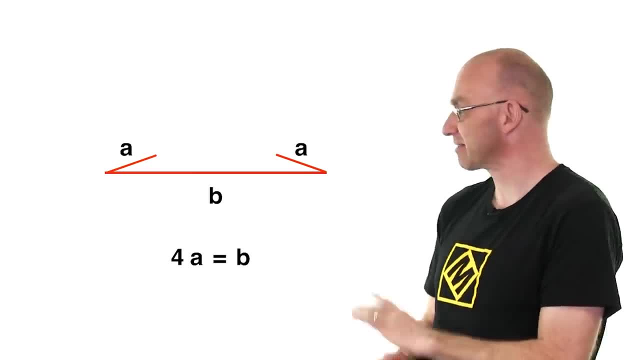 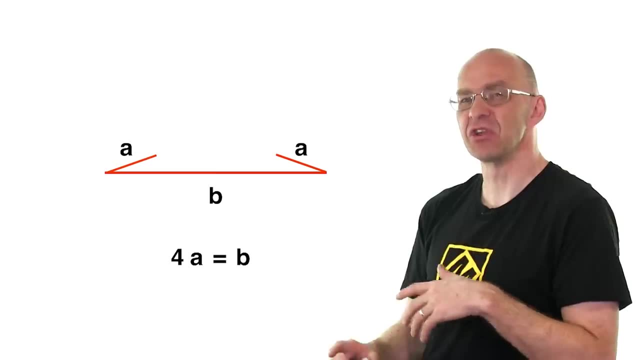 So just forget about it. It's a big no. it's not going to work right, So it's pretty wrong. It's pretty wrong, But it can get even wronger, So let's just have a look. at like any triangle whatsoever. 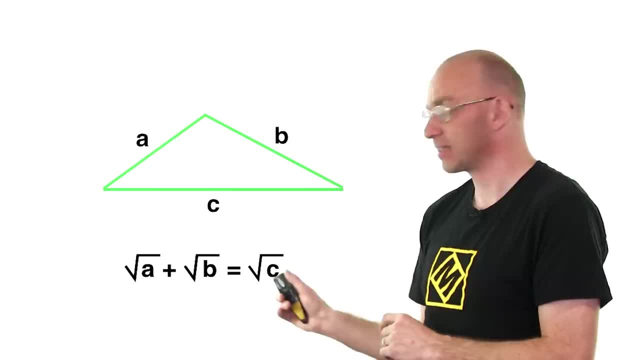 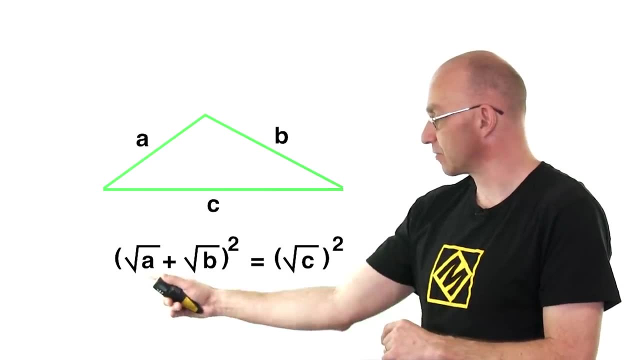 and have a look whether you can actually get: square root of A plus square root of B is equal to square root of C. So again, to get rid of the square roots, we just square the whole thing right. So square here. So now what do we get here? 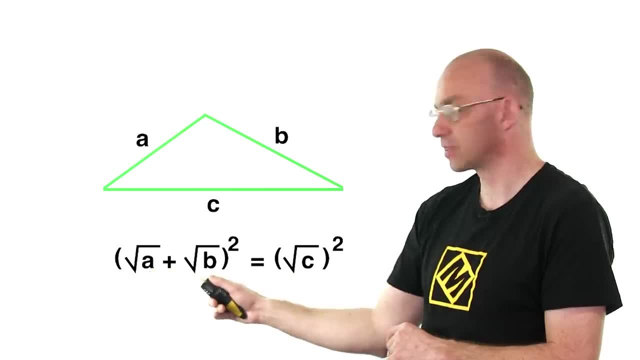 We get the first time's guy squared Plus two, times. this times that plus okay. So what's this? one squared A, A, And then we get plus Two: square root of A, square root of B. Yep, that's right. 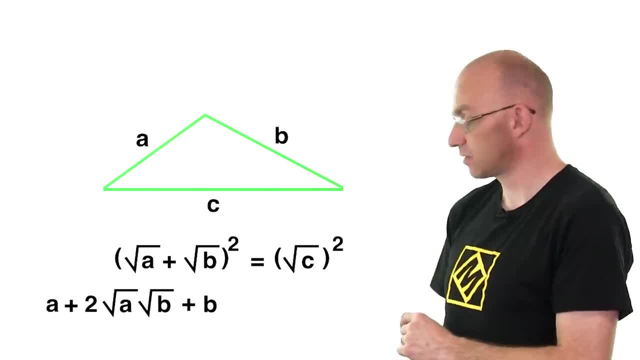 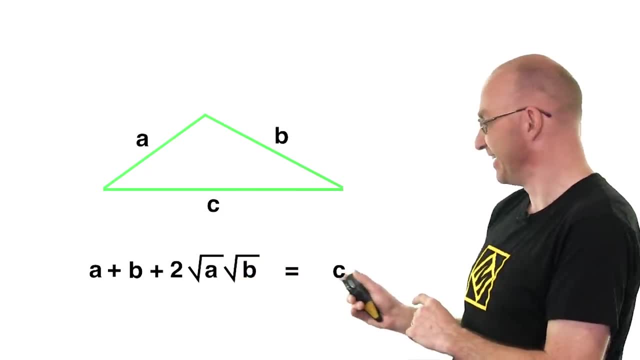 And then the last one is B, B, okay. And then on this side, C, C, okay, cool. Now just rearrange this a little bit and you get A plus B plus something C, right? So basically what this says is that C is a little bit longer. 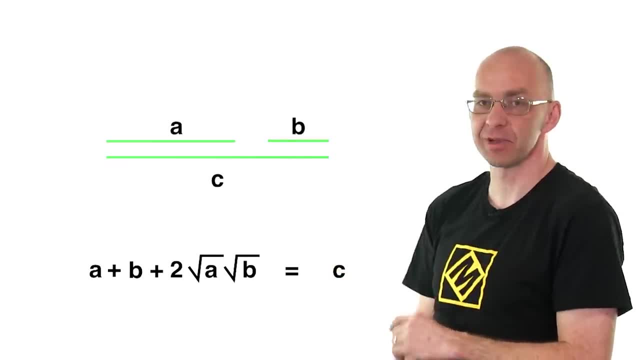 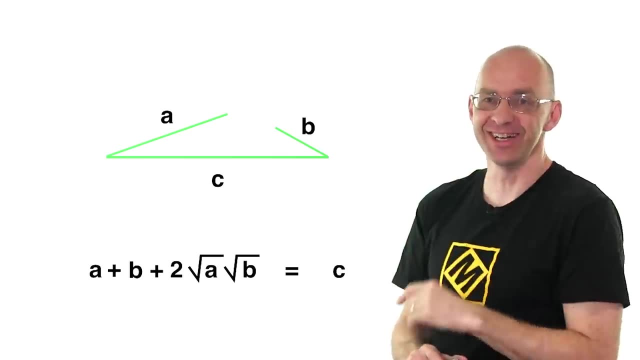 than A and B put together. So there's A, there's B, and C is a little bit longer. And again it's pretty obvious: you can't make any triangles out of this right, So it's pretty wrong. Also, I mean this is isosceles triangles in the plane. 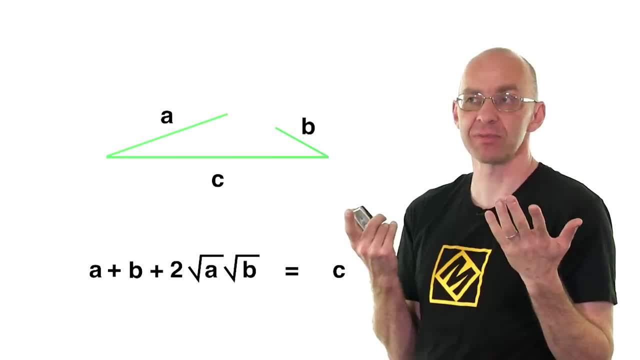 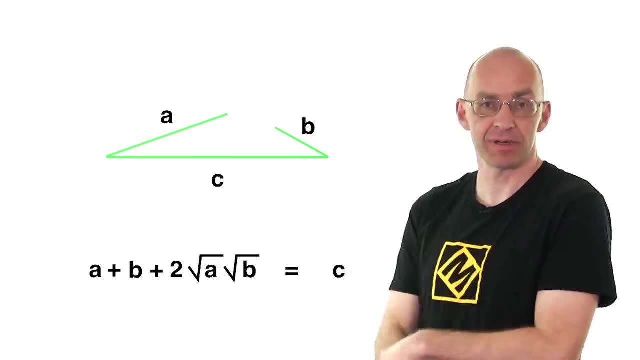 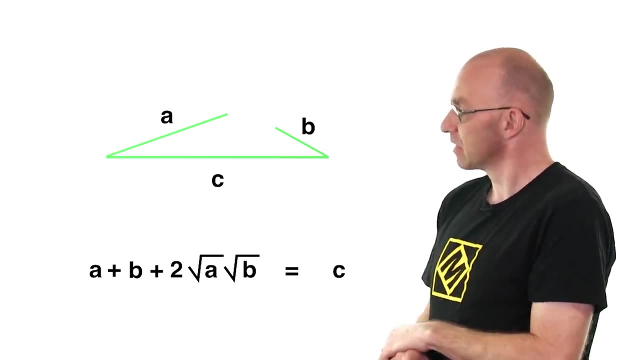 What happens if you actually kind of look at triangles, maybe on a sphere or on a weird surface or anything like this? Can you actually get like the Scarecrow's theorem or Homer's theorem to work anywhere? Well, hmm, Well, in the plane. what really kills this one? 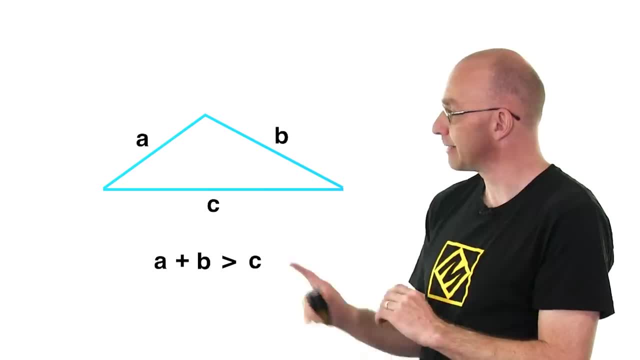 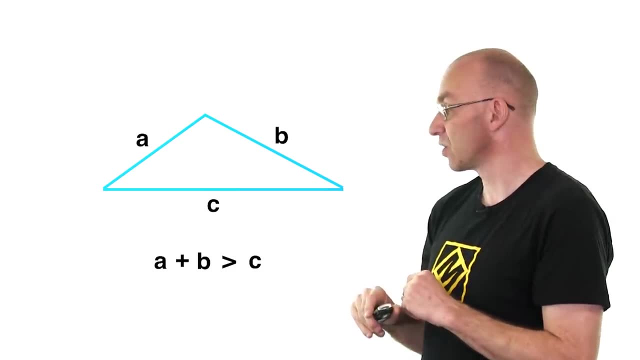 here is the fact that in any triangle, A and B always add up to something that's bigger than C, And basically the Scarecrow theorem contradicts that right. So what we're really aiming for is a world in which this guy here is not satisfied. 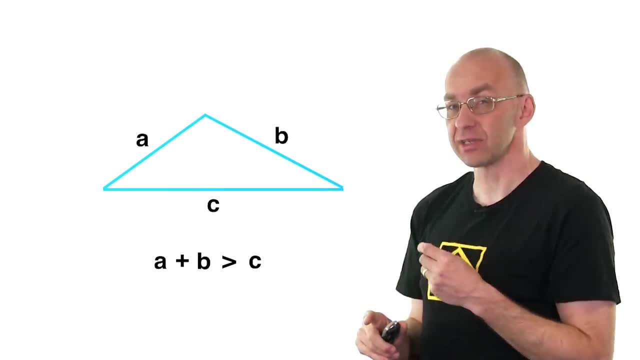 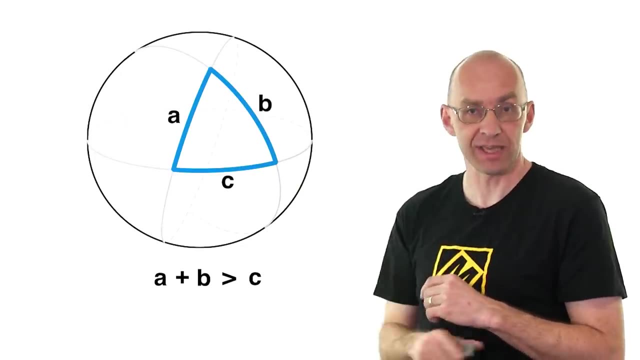 It's called a triangle inequality, okay, And it actually turns out that it's very hard to find anything reasonable where this doesn't hold. So, for example, if you look at triangles on a sphere, they all satisfy this. So even on a sphere, the Scarecrow's theorem doesn't work. 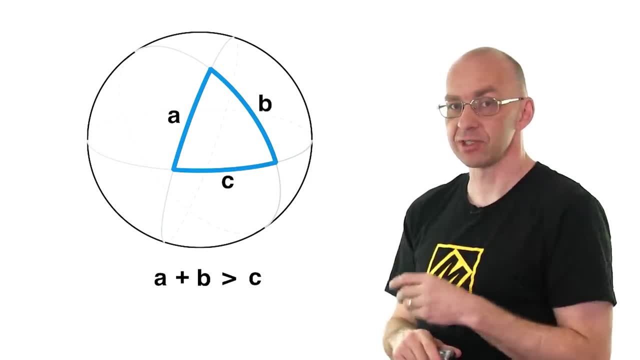 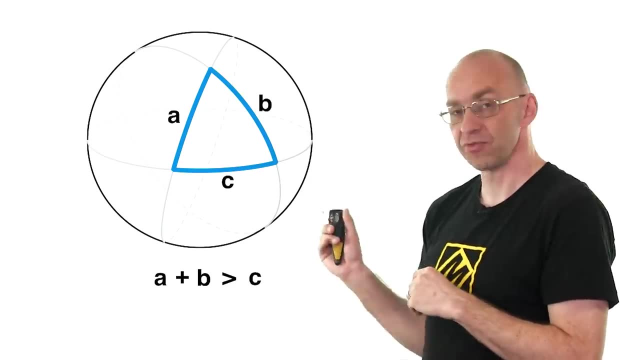 or the Homer's theorem doesn't work. But you know there's lots of mathematicians out there who know about lots and lots of really really strange worlds, So maybe one of you has an idea for a strange world where we can actually make this work. 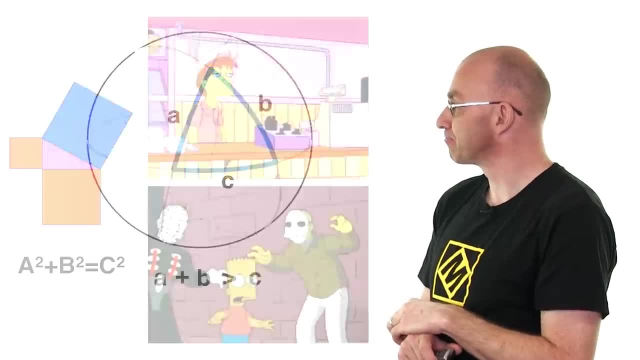 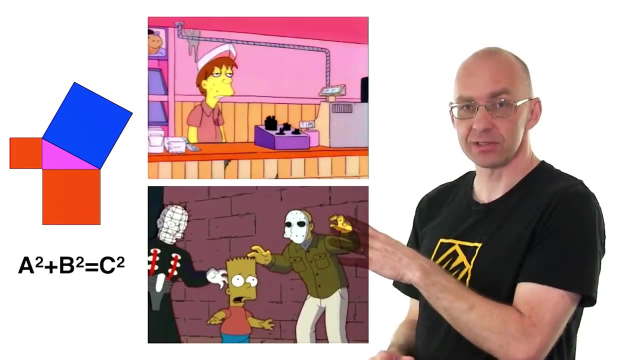 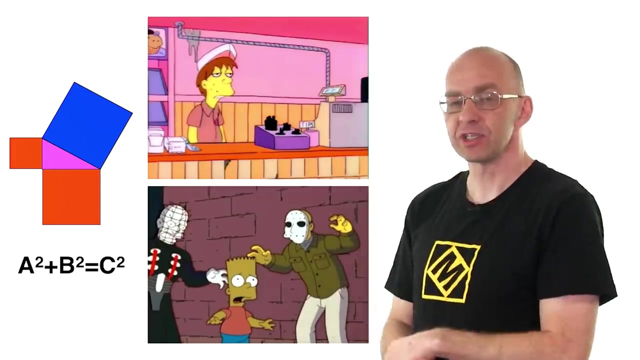 maybe just in one instance. Okay, Right Now I actually also started digging to see whether I can actually find Pythagoras. Pythagoras actually does pop up in The Simpsons. I know of two instances And actually one of your missions is going to be. 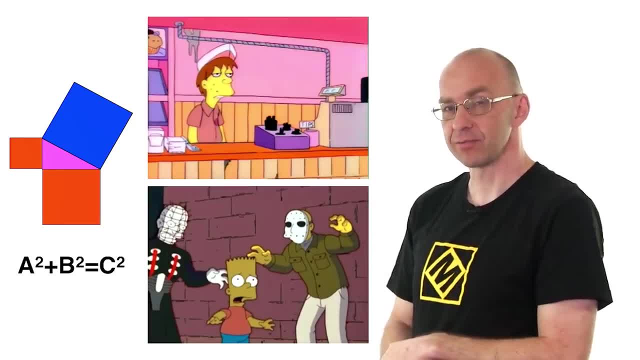 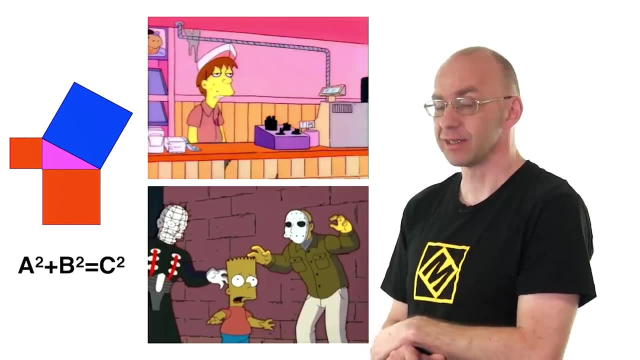 to figure out where exactly in those clips Pythagoras pops up. Maybe some of you actually know of other instances of Pythagoras or the Scarecrow or Homer's theorem in The Simpsons that I'd really like to know about it. Even other movies, other episodes, other TV episodes. 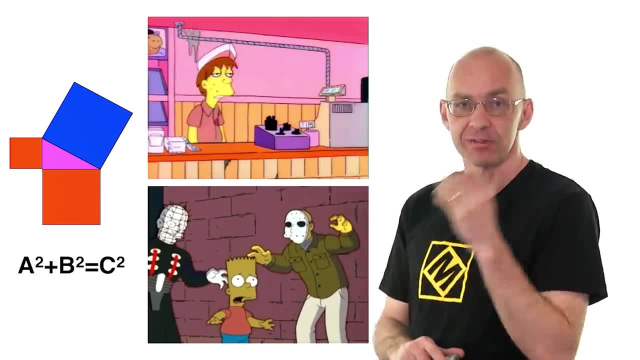 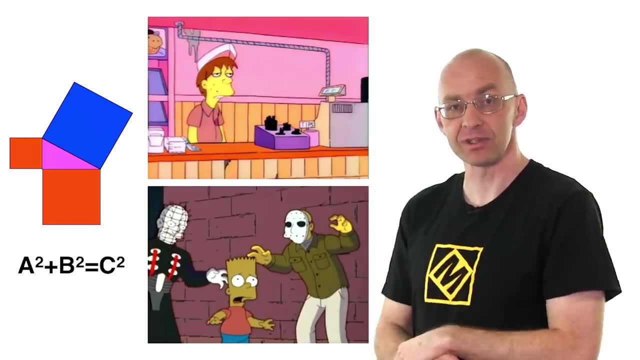 I'd be really interested in finding out And for The Simpsons lovers among you, as I said before, you know pinpoint all the episodes where these things are from. Okay, Let's have a look at the first clip and see whether you can see Pythagoras somewhere in there. 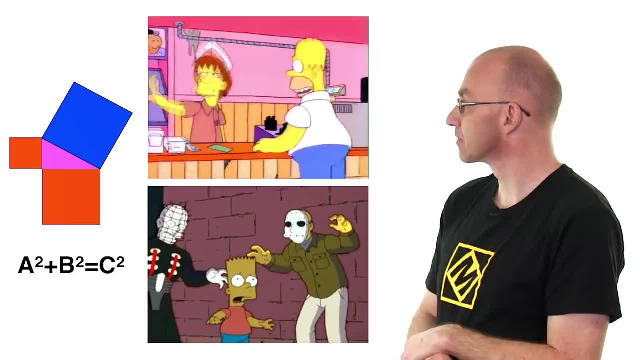 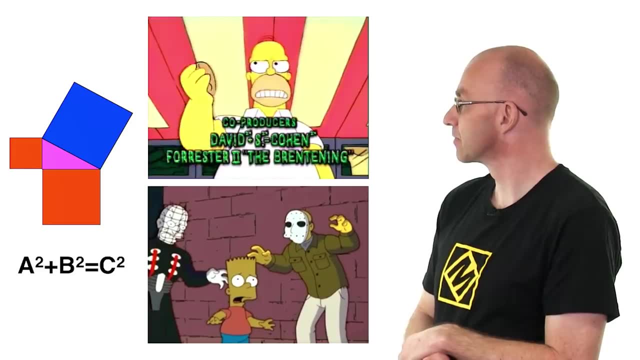 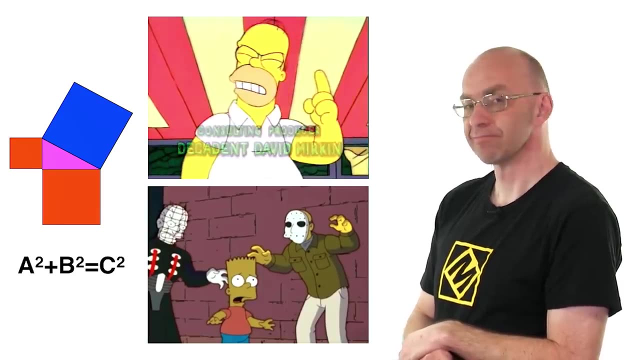 I want a colossal doughnut, just like the one on the sign Doughnuts. That's false advertising. Sorry, sir, No refunds. I paid for a colossal doughnut and I'm gonna get a colossal doughnut. That's a tough one.